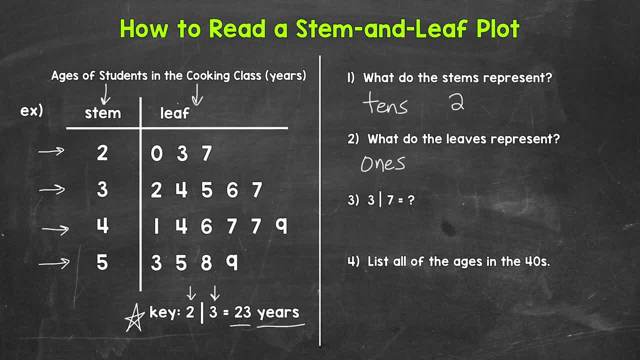 Think of the stems like this: The stem of two is in the tens place And then the leaves will be in the ones place. That's the twenties, And then we have the thirties. So a stem of three and then the leaves in the ones place. 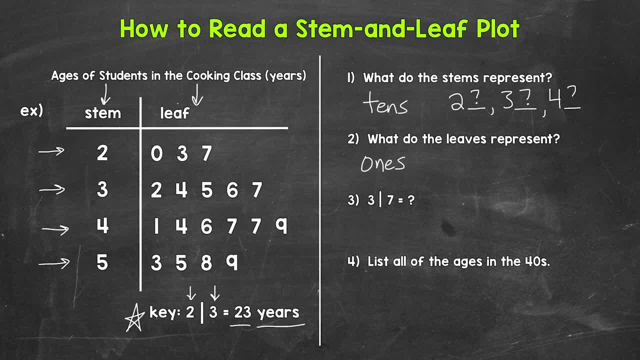 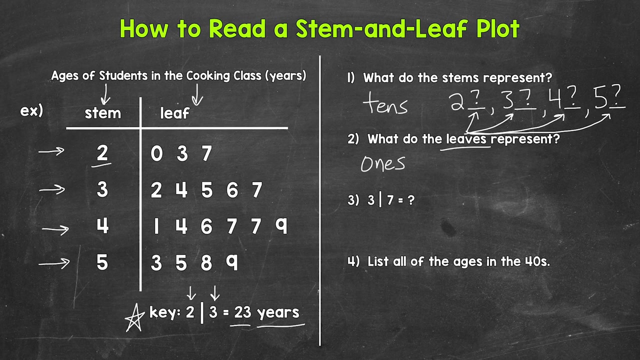 Then we have the stem of four with the leaves in the ones place And then the stem of five with the leaves in the ones place. So the leaves will be the ones place. They will fill the ones digits here. Let's put this all together here and look at the stem of 2.. 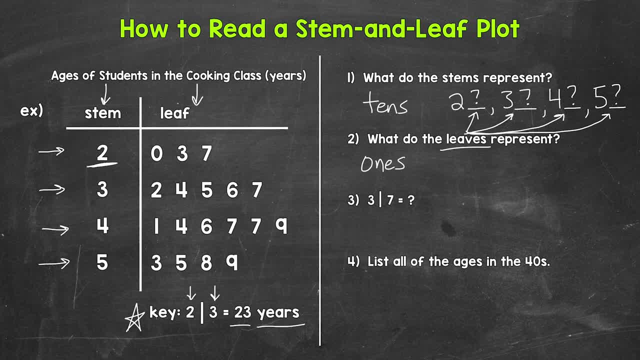 So if we have the stem of 2,, let's move over to the leaves, where we have 0,, 3, and 7.. Now, if we put the stem and those leaves together, we have 20,, 23, and 27.. 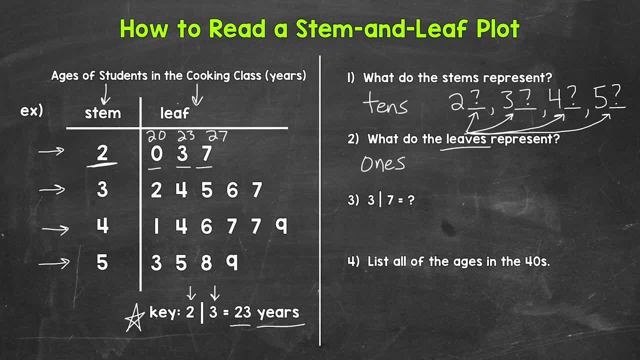 So those are all of the ages in the 20s And, looking at the stem and leaf plot, we have a 20s group, a 30s group, a 40s group, a 50s group. So everything is organized. 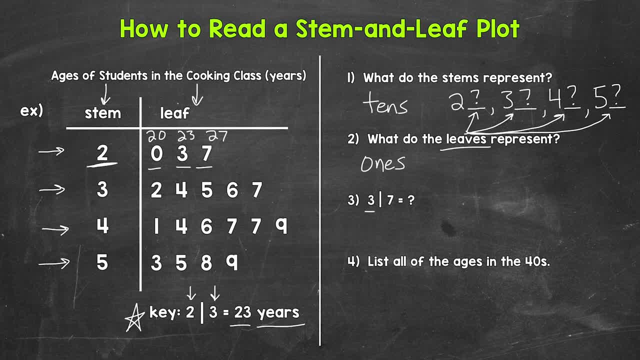 Let's move on to number 3, where we have a stem of 3 and a leaf of 7.. So what does this equal? And if we look at the stem and leaf plot: stem of 3, leaf of 7.. Well, let's put that stem and leaf together. 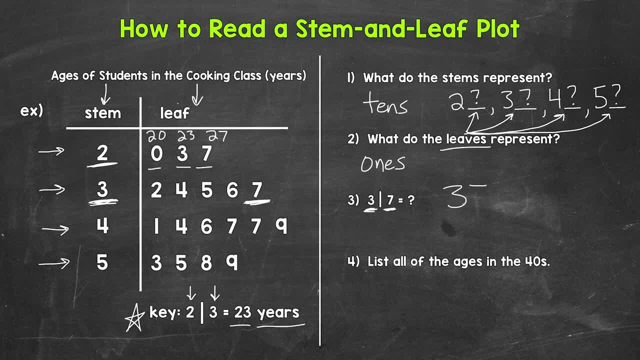 The 3 is going to be in the tens place and then the 7 is going to be in the ones place, So that gives us 37. So again, just putting that stem of 3 together with that leaf of 7. And that gave us 37.. 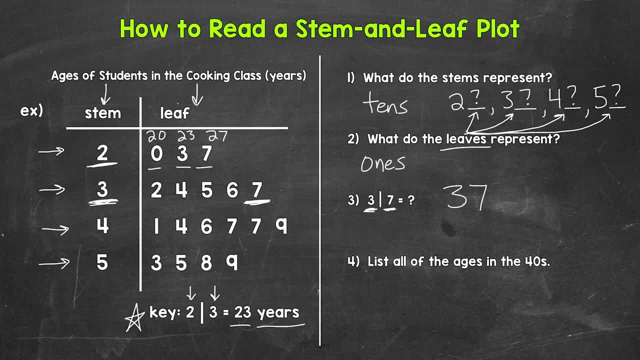 Lastly, let's move on to number 4, where we need to list all of the ages in the 40s. So let's take a look at the stem of 4 and then these leaves. So let's put that stem together with all of those leaves.